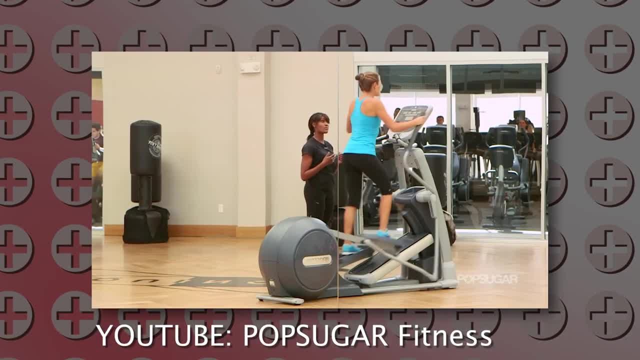 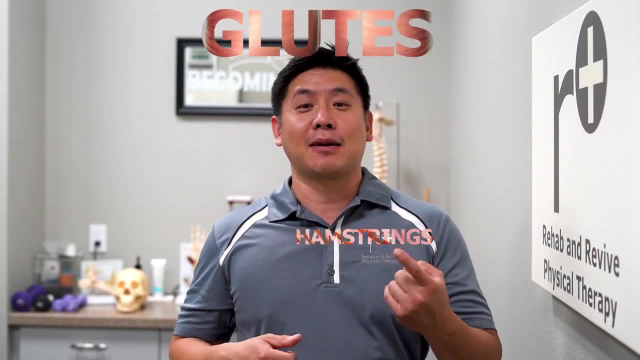 it keeps a regular form. If you do it correctly, it gets the right motion. You're working on important muscles and important muscle groups, like your glutes and your hamstrings, if you do it correctly. So stay tuned. I'm going to show you how to. 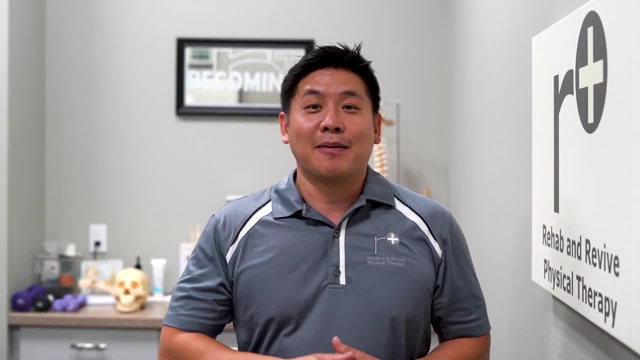 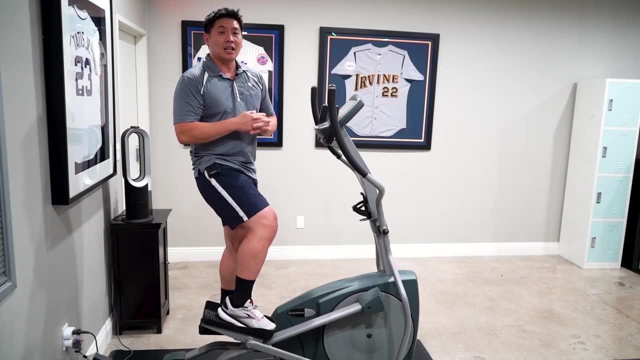 swing the elliptical machine, Swivel on that machine and do it well Good, All right, we're back. We've got our elliptical machine. Let's talk about how to use this correctly. A lot of people are using ellipticals. I see it at the gym all the time. 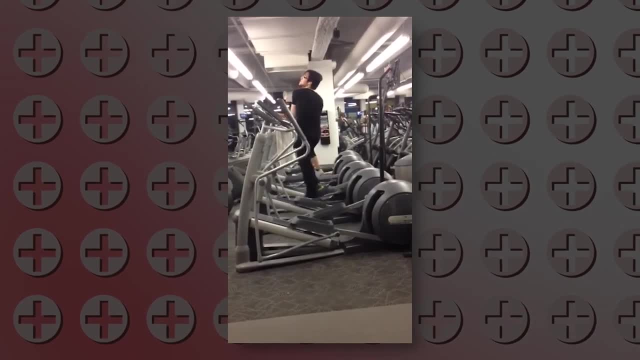 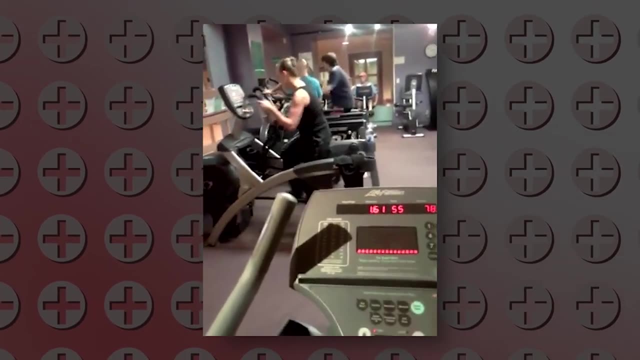 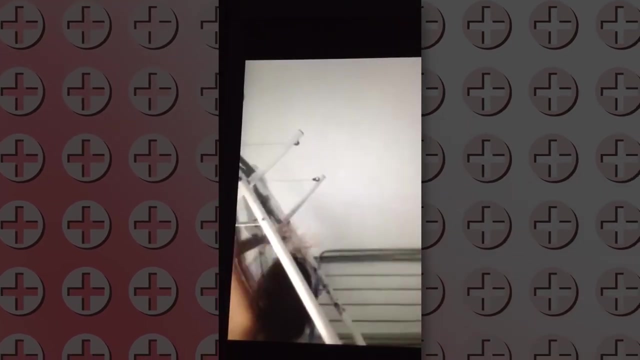 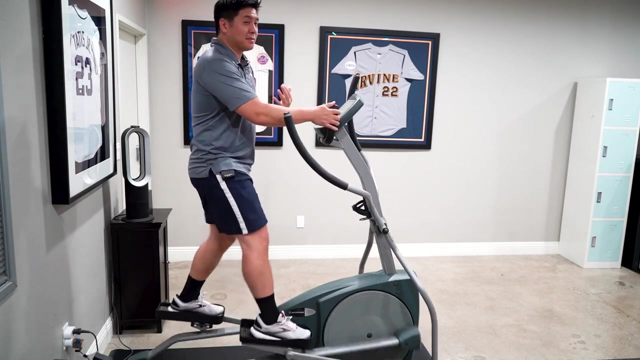 just incorrectly Swivel the arm and swing it all the way back to the middle. This is how they're doing it. They're either using the arms- It doesn't matter to use the arms- or just hold place. It doesn't matter to me. I think sometimes people like that little extra assistance. 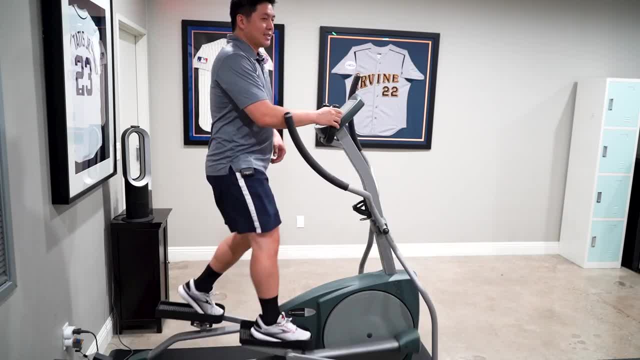 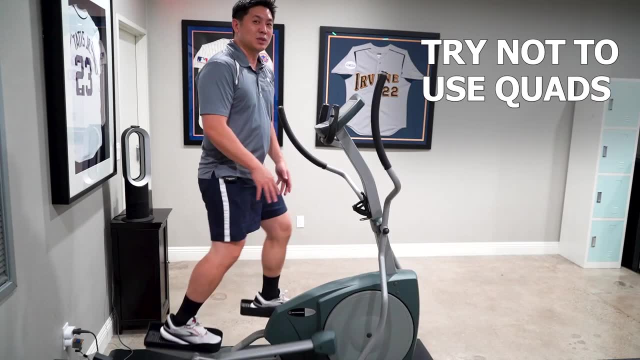 because they're pushing with their arms and pulling. but a lot of people do this. They're really at the front of this pedal and they're lifting their heels. Now, that's a lot of quads and that's really what we're trying to avoid. We want to get our hamstrings and our glutes involved. 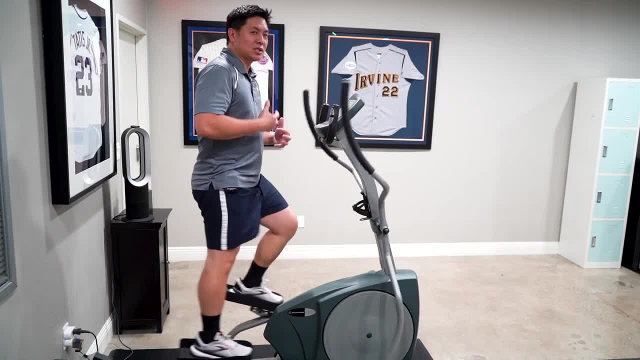 and really I like to tell people it's like a giant heel. So we're going to go ahead and do that: Swivel the arm and swing it all the way back to the middle heel slide. we have a great exercise. the heel slide, it's essentially the same thing, you're. 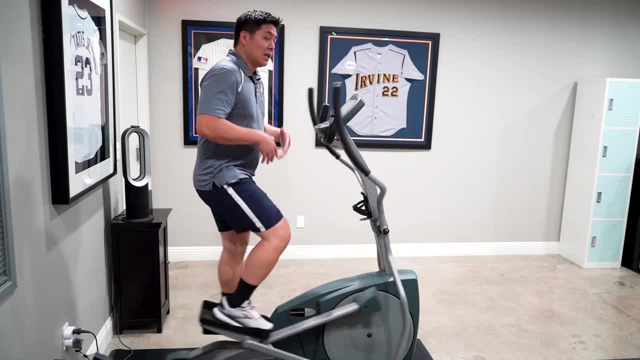 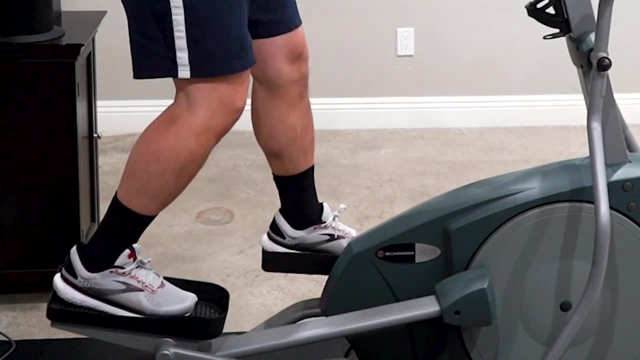 just doing repetition and repetitions over of it. so here's the right way of doing it. what you want to do is you want to sit in the back and you want to jam your heel into the back of the pedal, and then you want to pull, you want to claw or you want to think of like a mechanical crane. 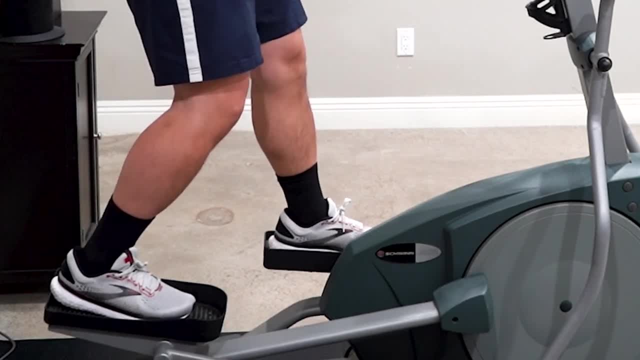 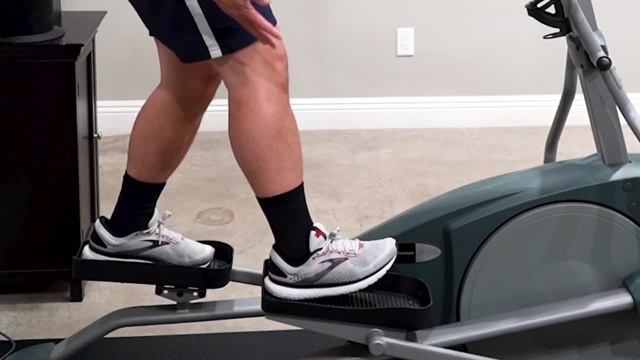 where you're dragging it through and pulling. dragging it through and pulling- this is what it looks like you're trying to. i'm exaggerating this part. i don't actually lift my toes, but i want you to get the idea that i'm pulling with my hamstring here and then, as i get up here, the 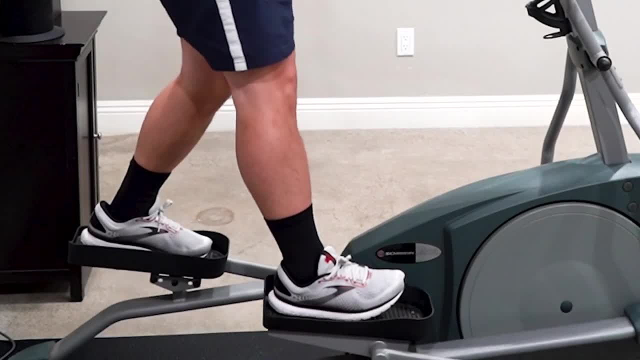 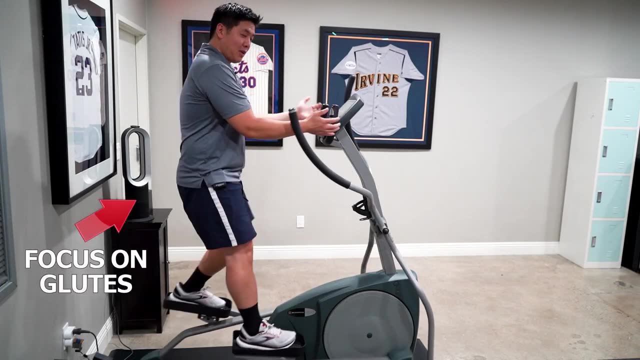 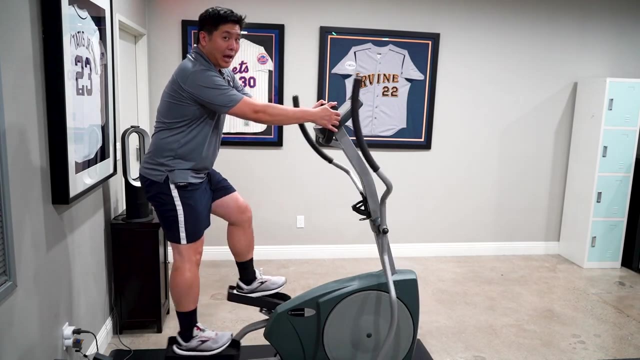 other hamstring, my left one right now pulls through, so it's pull, pull, pull, pull. and so this is i kind of like leaning back just a little bit, almost holding the handles here where i'm. this is the motion. i just want you to show you that i don't really do that, but we'll do a real time one. 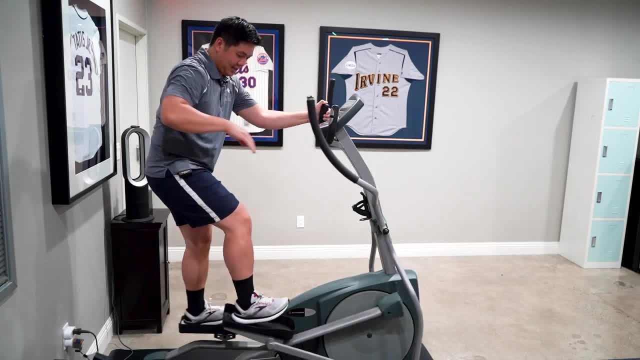 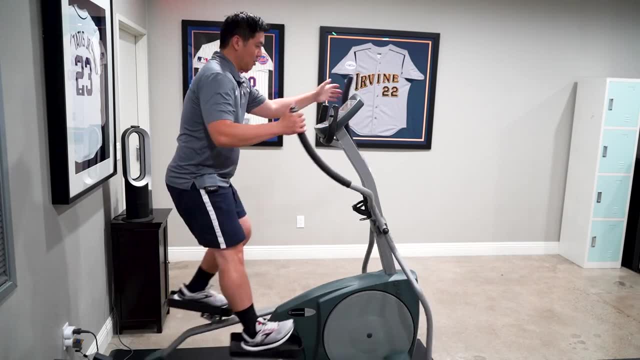 in a second, but i'm dragging it, dragging it, dragging it. the other one's going now dragging it on the right, left one's dragging it, and that's what i want you to get. so here's what it would look like for me. so i'm leaning back. 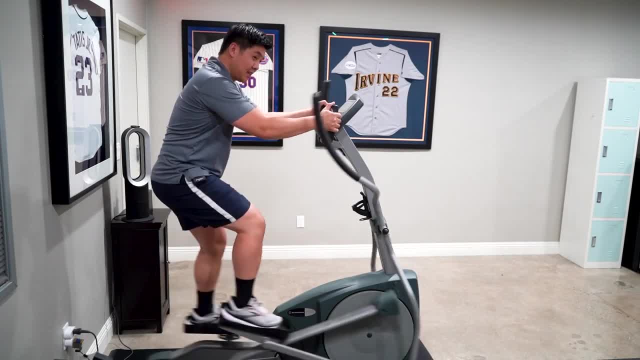 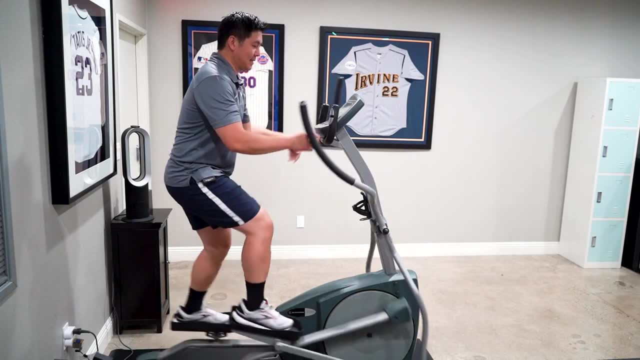 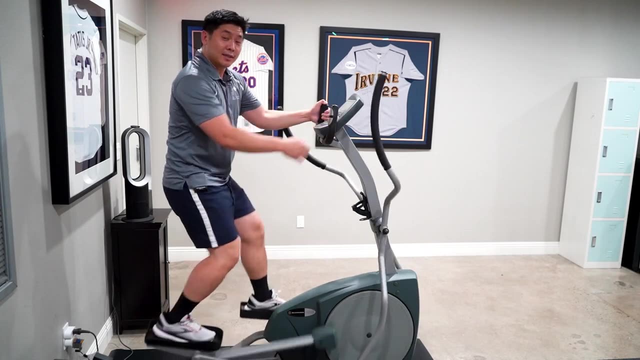 using that so and so we can go fast, we can go slow. i like to tell people we're still aligning our posture, our throat, our sternum, our belly button and our pubic bone in one line, so happy enough to be able to do that. people are so excited about this- almost impossible to do. 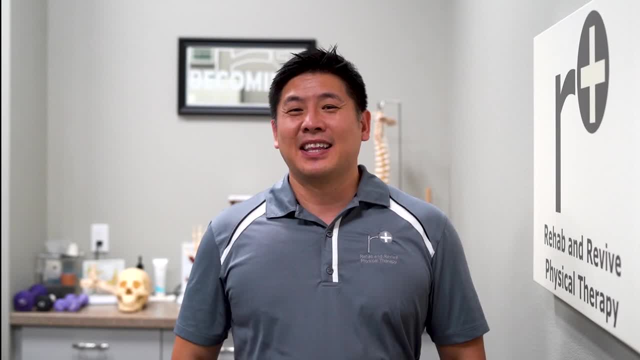 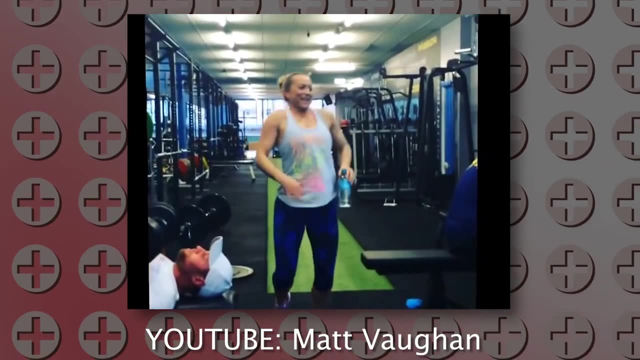 the whole thing. you can get this thing done in just a couple of minutes, so i hope you enjoyed it. i hope you did, and i hope you will like it so much as you do. and i hope you did, and don't forget to like the video and subscribe to my channel, because i'm going to make a video of you rowing. 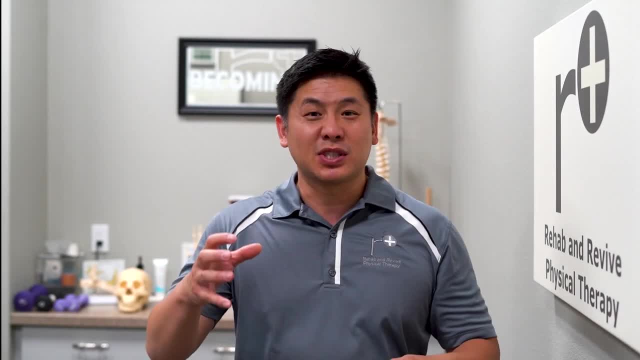 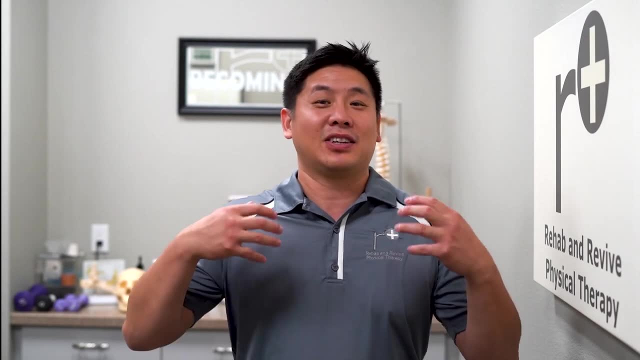 down to the studio and then pedaling on the elliptical, we'll get right back to the studio. all right, we're back. boy, my glutes, my hamstrings, they've been worked. let's go that workout. you can get sore. i expect you to get sore in those areas, so, but make sure, this is the 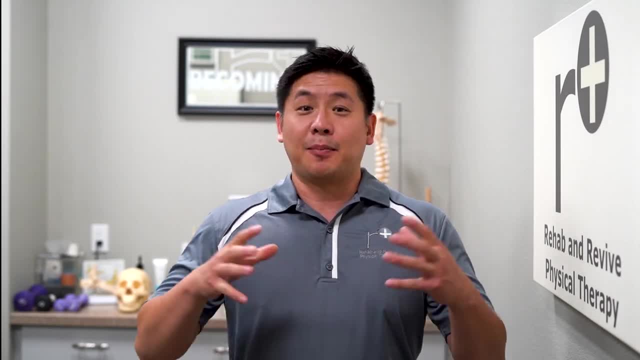 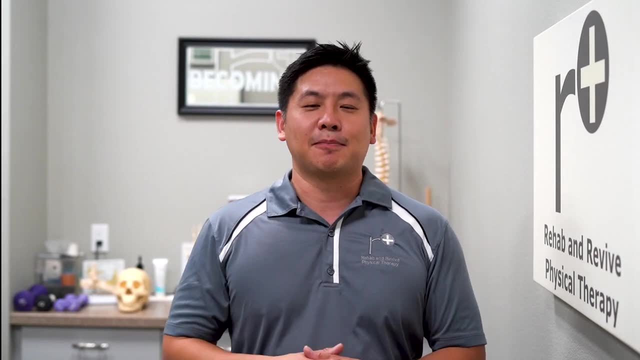 right exercise for you. you've checked with your healthcare professional and, but otherwise i think it's a great cardiovascular low impact exercise for those of you who have other dysfunctions and many lower extremity parts. uh, if you like what we're doing and you have any feedback, try these. 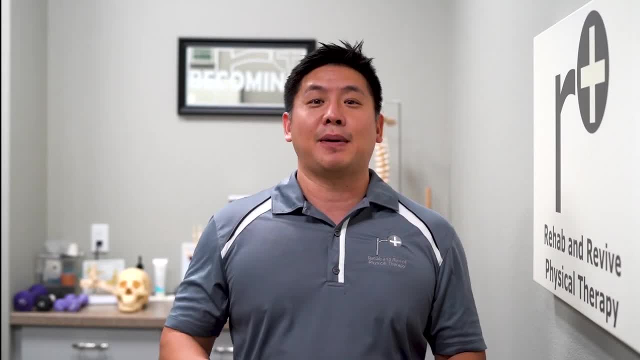 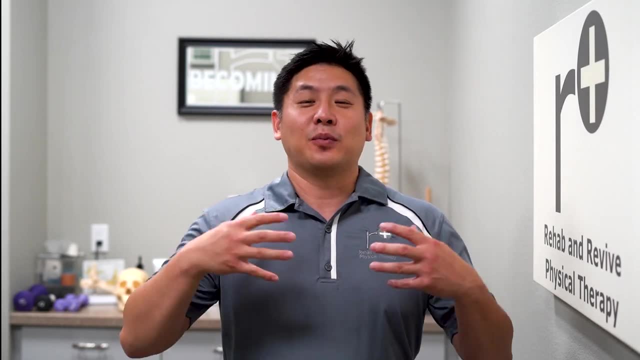 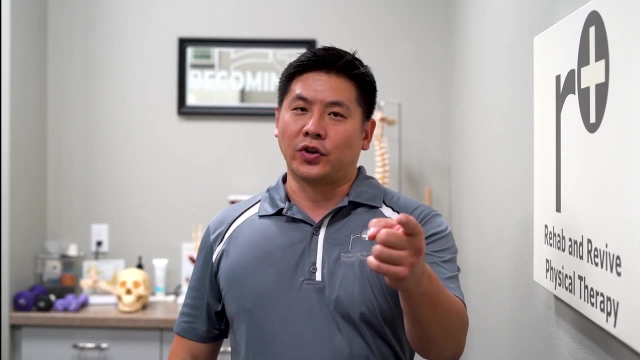 exercise. try this one specifically. leave any comments and feedback below. we always like this if you like the video and, of course, we love your support through this time, and we enjoy giving you out new information weekly, so subscribe below. i'm dr lin. remember we heal smarter, not harder.